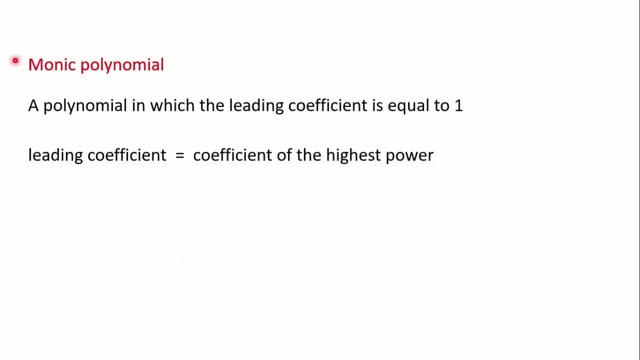 In this video we are going to learn about monic polynomials. So let us begin with the definition. A polynomial in which the leading coefficient is equal to 1 is called monic polynomial. Now you might wonder what is this leading coefficient means? So leading coefficient means a coefficient of the highest power, Just like if we have a polynomial here 2x squared suppose. 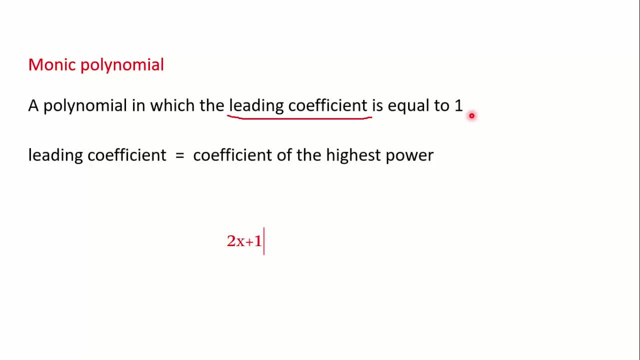 Or 2x plus 1.. This is a polynomial and in this the highest power of x is 1 and here leading coefficient is 2.. So in this polynomial the leading coefficient is 2, or we can say the coefficient of the highest power is 2.. So a polynomial in which the coefficient of the highest power is equal to 1 is called monic polynomial. 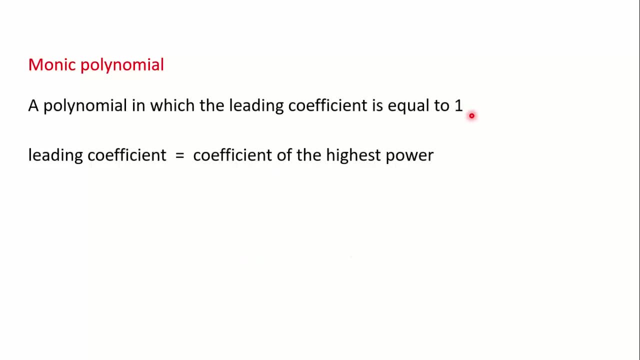 This can also be called monic polynomial. This can also be the definition here. Now let us see some examples so that we can understand more. Okay, so here we have: on this side we have some polynomials which are monic polynomials, and on this side these polynomials are not monic polynomials. So let us see how they are monic and how they are not monic. So begin with this one. This polynomial has the highest power, 2.. Okay, so it's a quadratic polynomial and you can. 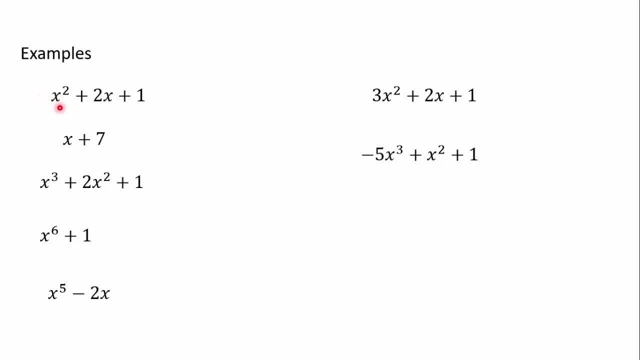 see, the coefficient of x squared is 1.. Okay, and here also this polynomial has the highest degree of 1, and here also the coefficient of x is 1, and in this polynomial also the coefficient of X cubed, which is the highest degree here, is: 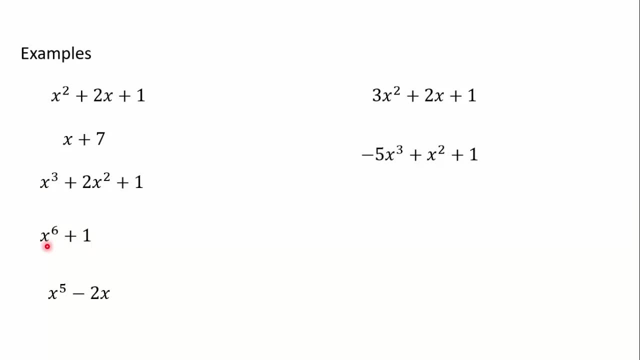 1, and here this one is sixth-degree polynomial, and the coefficient of x to the power of 6 is 1. so all in all these examples, you can see in all the examples the coefficient of the highest degree. here it is one. so these all are examples of monic polynomial, while coming.